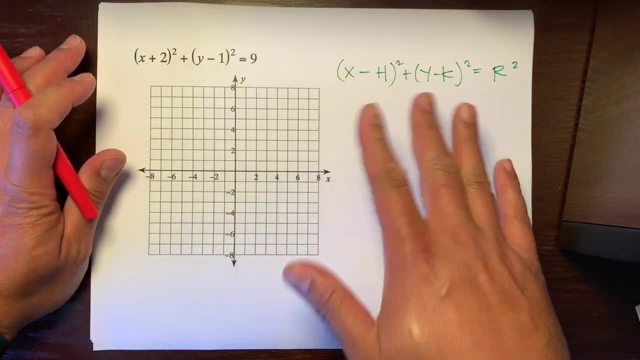 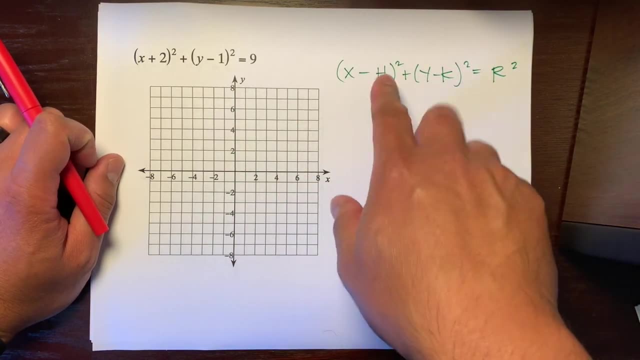 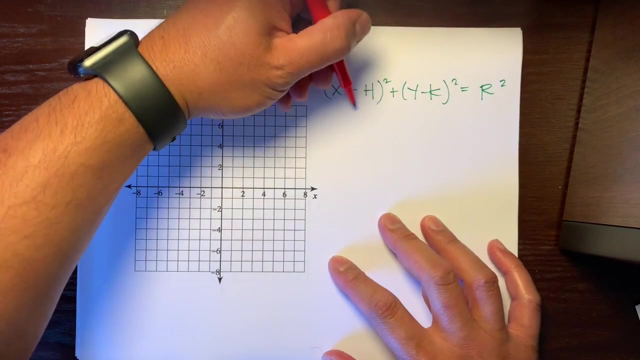 formed by using the Pythagorean theorem, And so that's why we have a square plus a square equals the other square. So here's: r represents the radius, and this h and k represent the center. So h and k are the center. Okay, so just remember that. this is important because 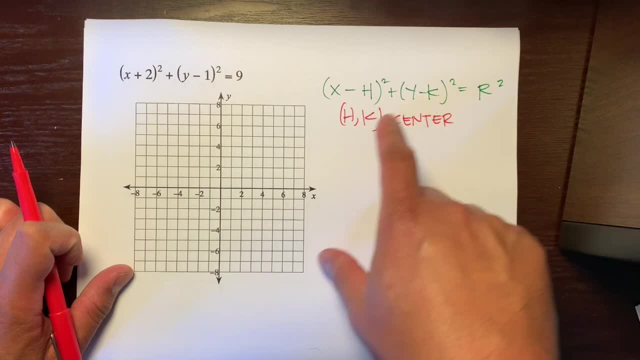 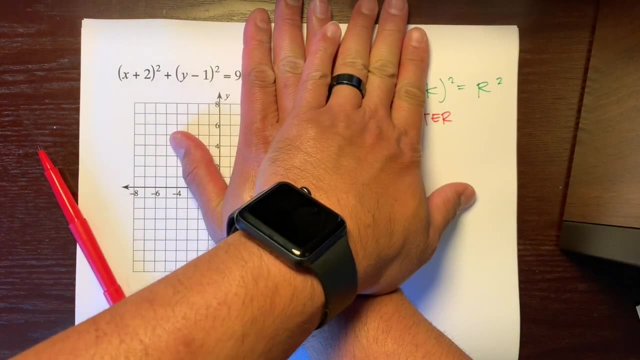 the center isn't negative h. the center isn't negative k, it's just h and k. So if we just cover that, that would be the x value of the center and this would be k would be the y value of the center. So if we just cover that, that would be the x value of the center. 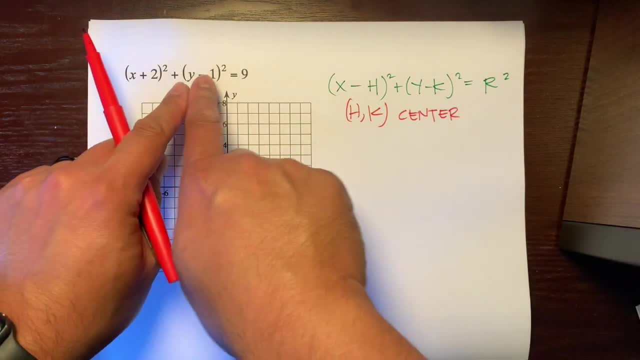 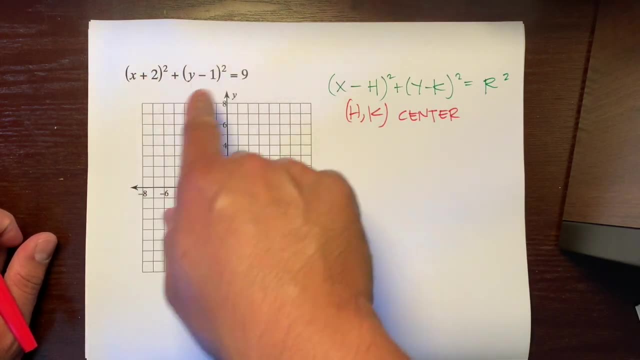 Okay. so let's look at this first example. Let's figure out what the center is. So if we plug this into the formula, okay, and so here's the first thing to notice, This is a plus, but the form is. 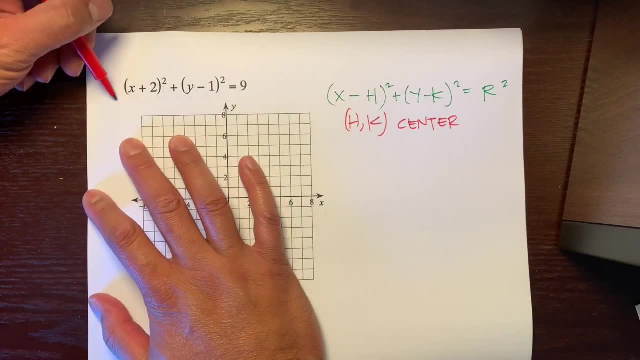 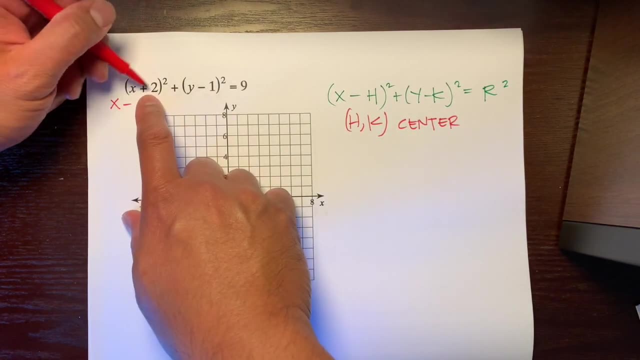 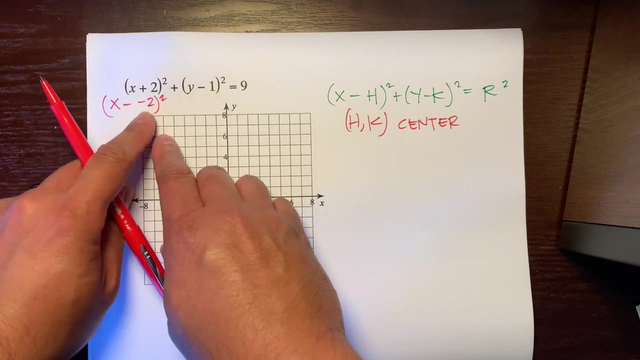 a negative. So what we're going to do is write it as x minus okay, because the form is a minus right there. And to get that pot, this plus two, we're going to write negative two Square. this is going to help us, because two negatives make a positive. So actually our h. 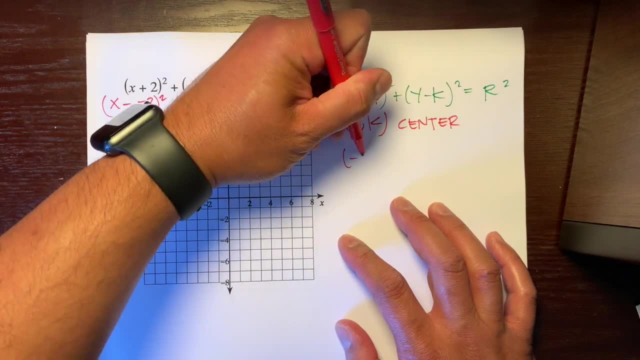 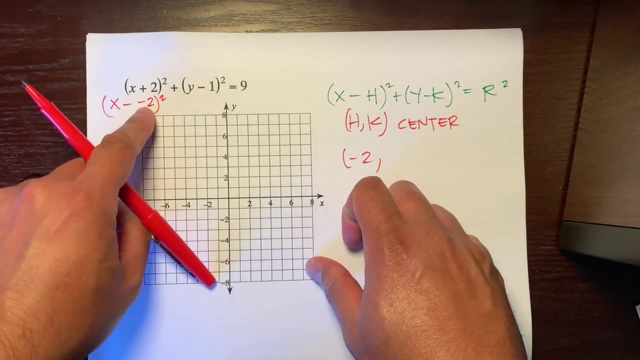 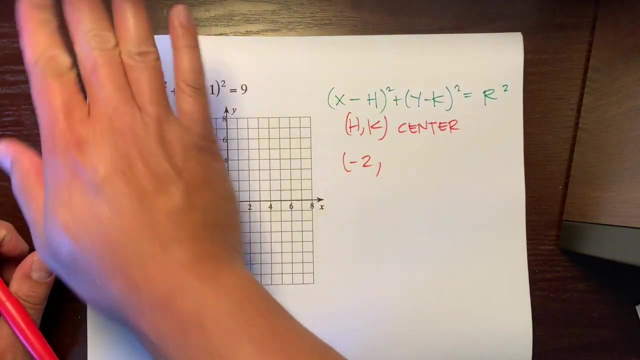 is negative. two, okay, because the form is x minus okay, and then the two negatives make a positive. So there's that. And then here, okay, and remember, we just take away, we ignore the negative and the y value would be positive one. So this right here. negative two: one is. 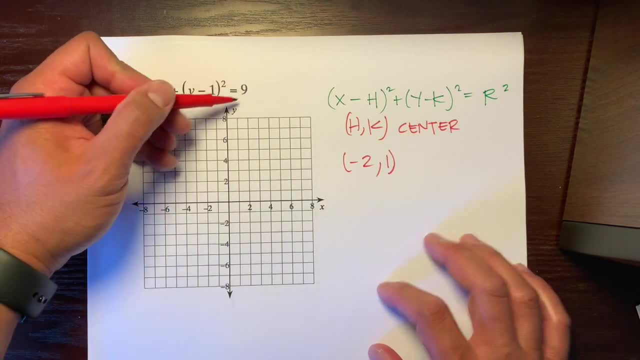 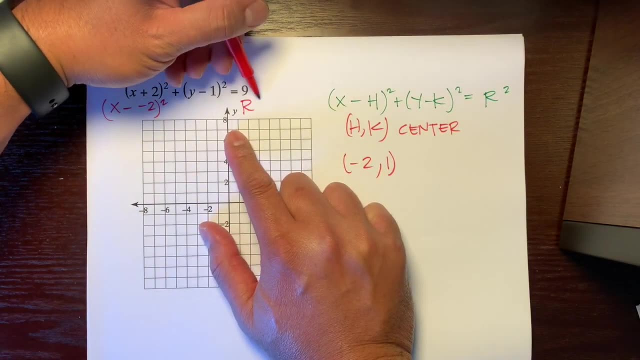 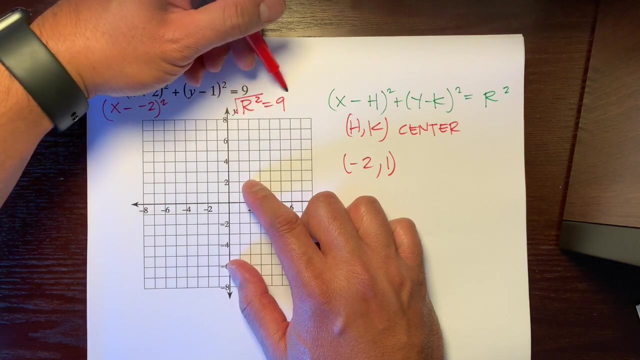 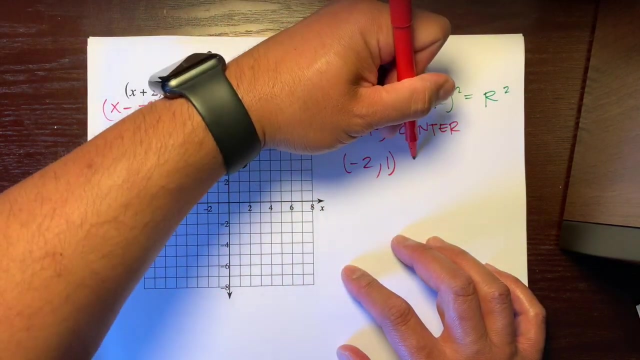 our center, okay, and then our radius. remember the formula is radius squared, okay, but we just want r. So if we did this, so this nine is equal to r squared. So the opposite of scoring something would be square rooting. So our radius would just be three, okay. So this is our center. 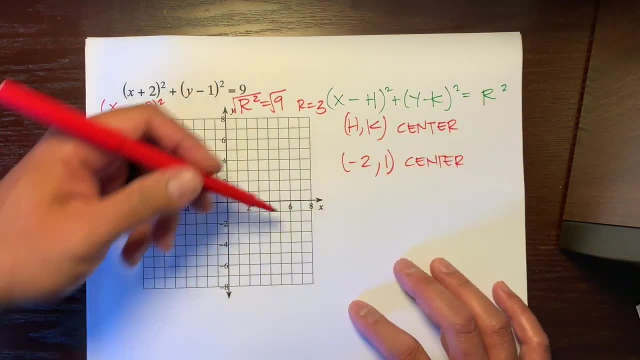 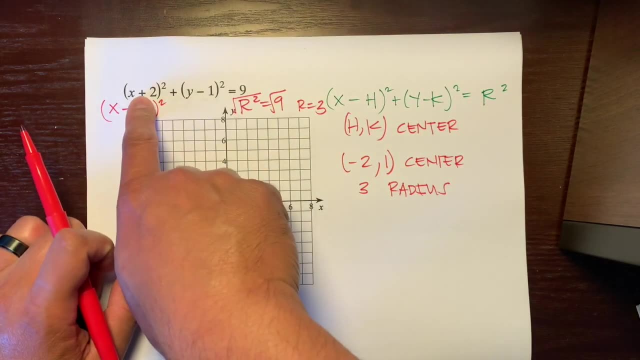 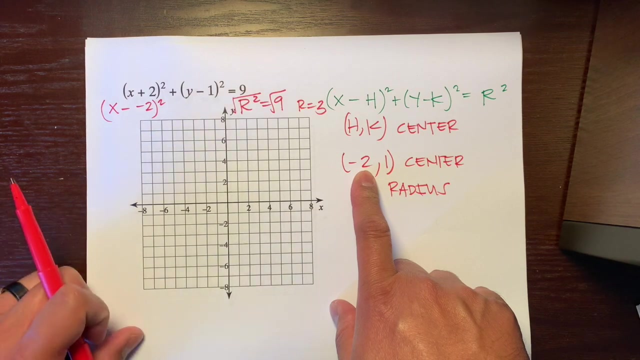 negative two, one and three, Okay. so the biggest thing is, when you have a plus, okay, write it as x, minus okay, and then to get that formula. So our center is at negative two. So remember, this is our x value for the. 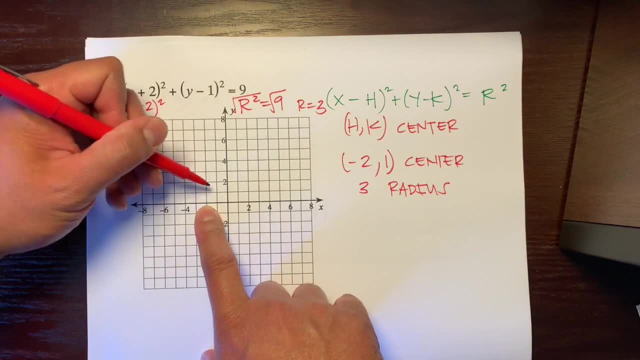 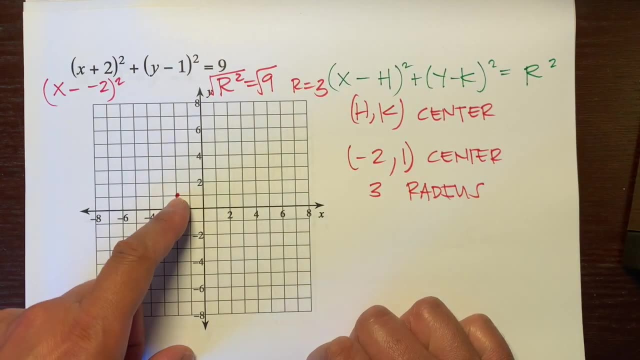 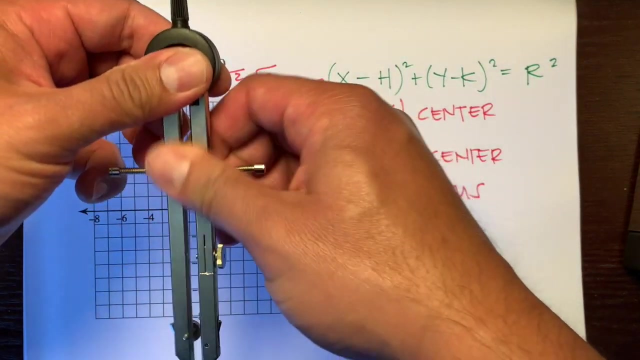 center and the y value is one. So we'll go negative two to the left and up one, And our radius is three. That means that every point on the circle is three units away from the center. So we're going to take our compass, And so here's the metal part, which will represent the 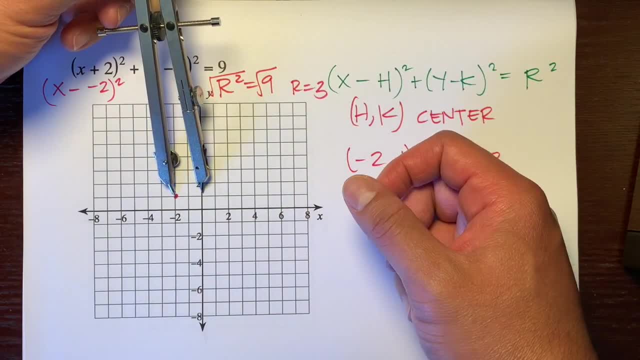 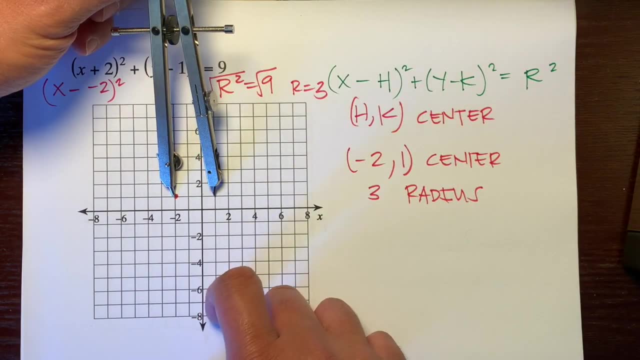 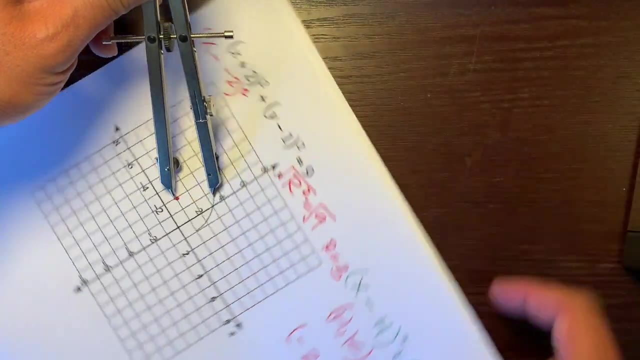 center, Don't push too hard because that'll hurt. And then we're going to open up our compass so that it's three units. So this from here to here represents our radius. okay, And it's a little easier to rotate the paper instead of rotating the compass, So I'm going to rotate the paper. 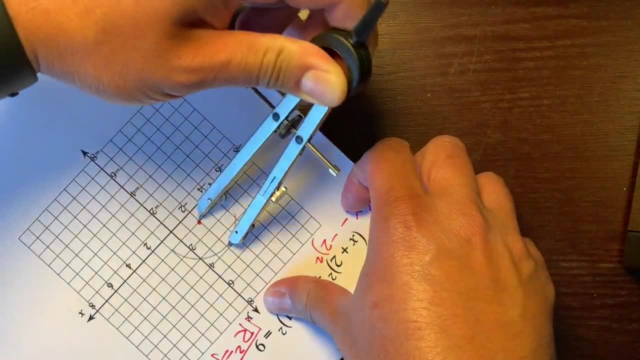 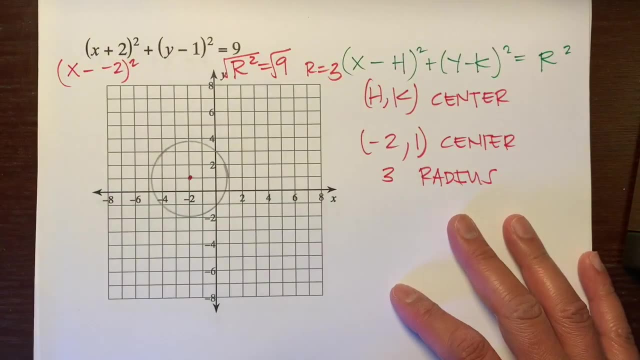 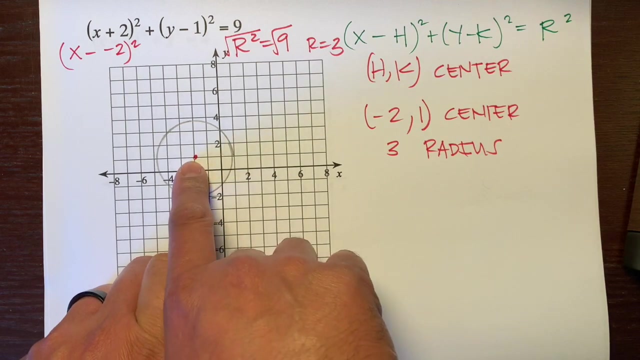 And it's still a little challenging, especially if it moved at the beginning. So then, rotate, rotate, rotate and there you go. So it's you know, my compass was a little off, moves a little, but if you look at it, here's our center, negative two, one, and our radius is three. 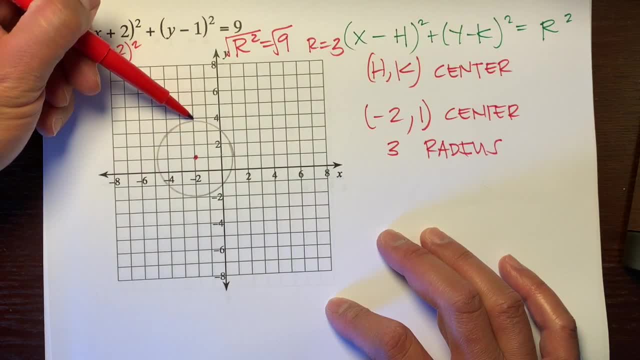 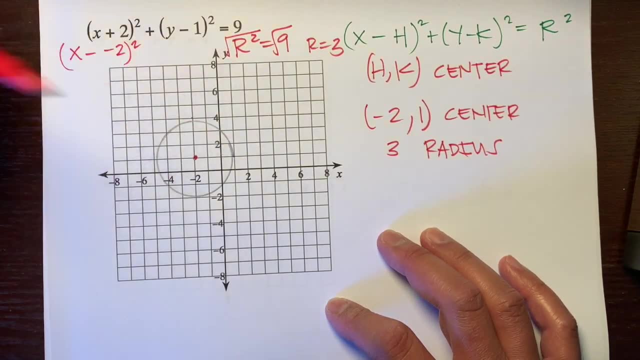 So this is. it should have gone a little higher, but this is three units away from the center. This is three units away from the center. Three units, three units. and if we kept on going, these radii would be three units away. So that's how you graph this equation. Let me give you 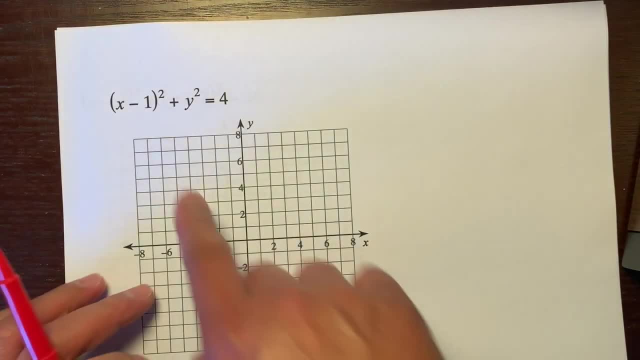 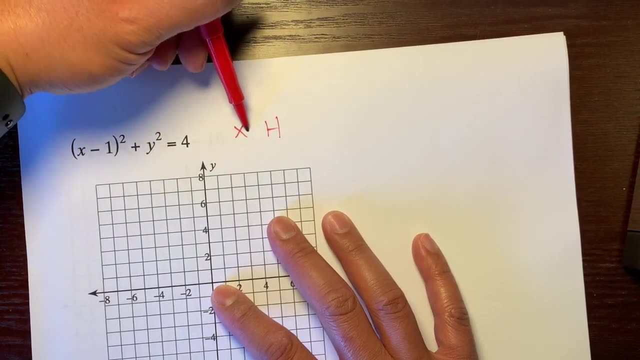 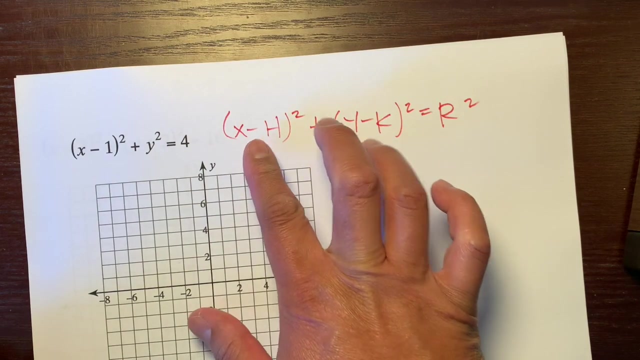 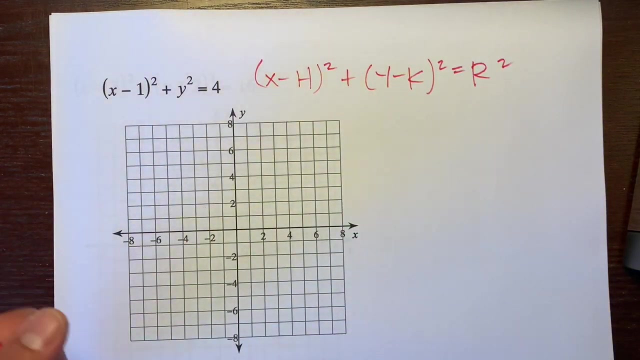 another example: Whoa. so let's rewrite that formula. Oops, x minus h squared plus y minus k squared is equal to r squared. So again, pay attention to those negatives, right there? Okay, so our center is: we'll ignore that: x minus, So our center is just one. 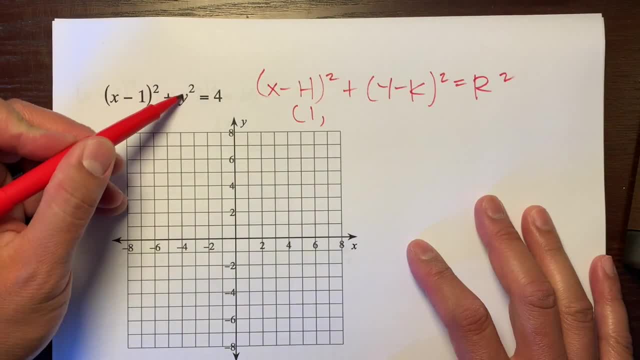 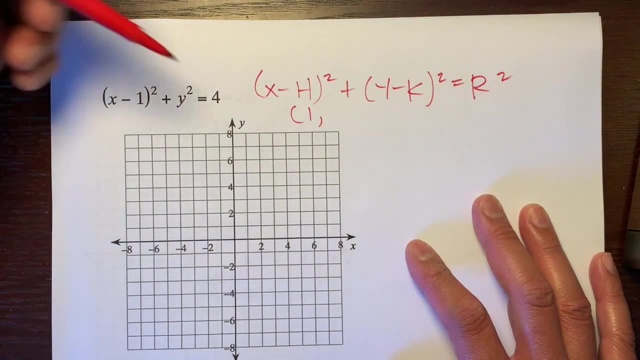 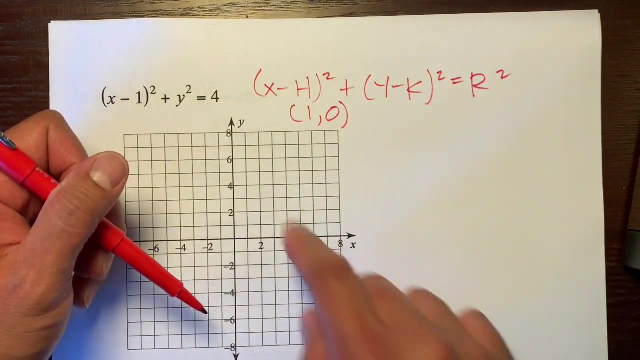 comma. Now, if you notice, here there isn't any number next to that y. So that means, if there's nothing, what's the value that represents nothing? Well, that's zero. So this is our center. And to get our radius okay, this four represents r squared, So we'll just set. 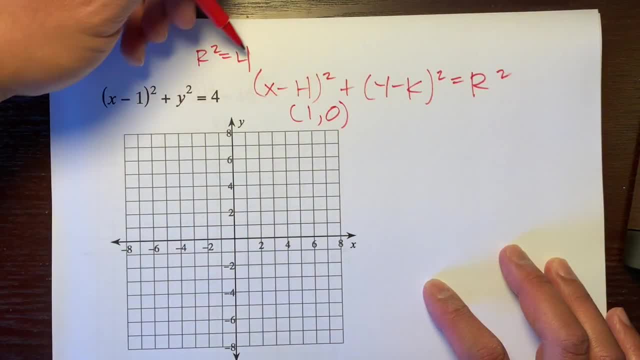 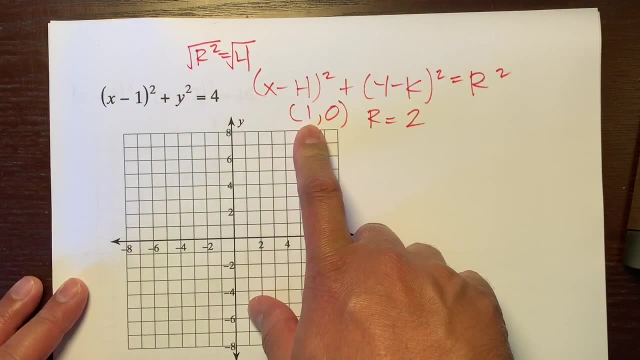 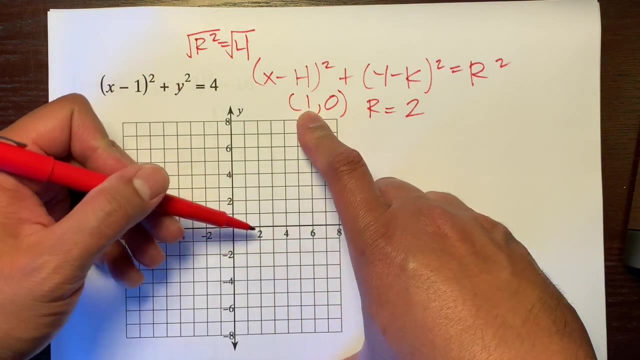 that r, squared, is equal to 4, and we'll square root both sides, and so r is equal to 2. so here's our center, here's our radius equals 2, so let's just plot it okay. so 1: 0, this 1 is our horizontal shift. 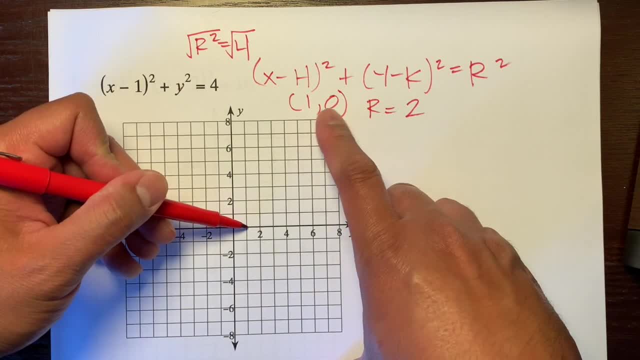 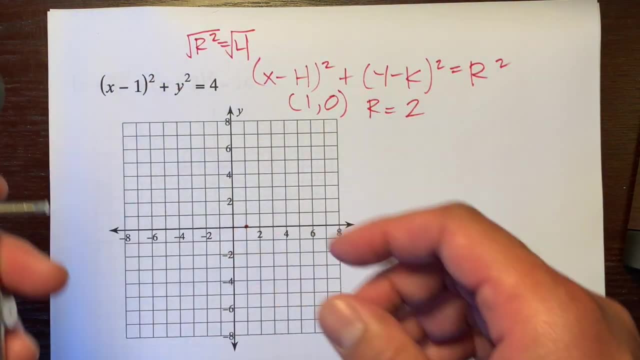 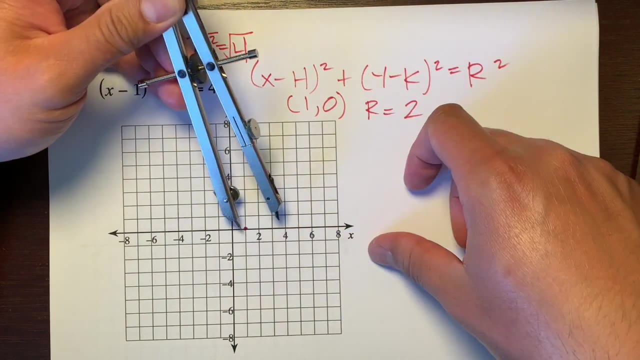 from the origin. so we're going to go right 1 and this says don't shift at all. so this is our center right here, and then we'll take our compass and open the radius. okay, so we're going to put this melt part right here, which is the sensor, on our sensor, and we're going to open the radius. so 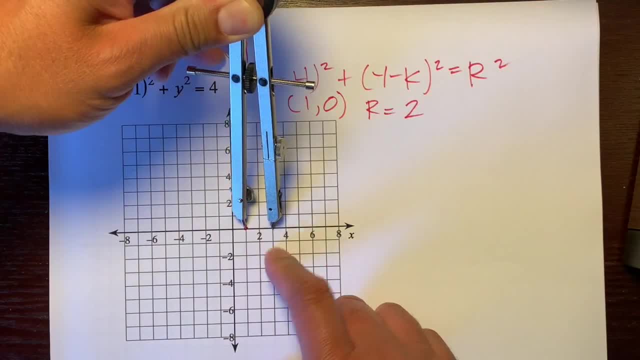 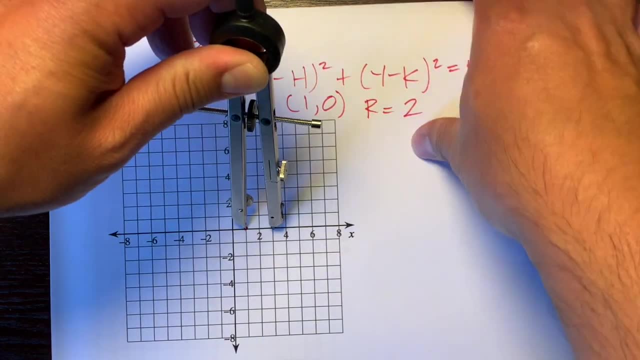 that it's two units. so from here to here is two units, and then let's see if i could draw a better circle than in the previous example. so let's rotate that piece of paper, rotate, rotate, and then we're going to take our compass, and we're going to take our compass and we're going to 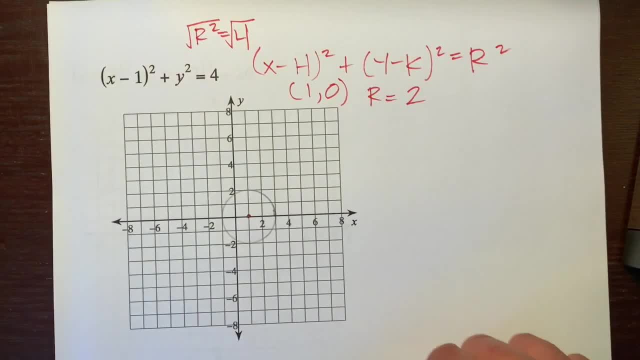 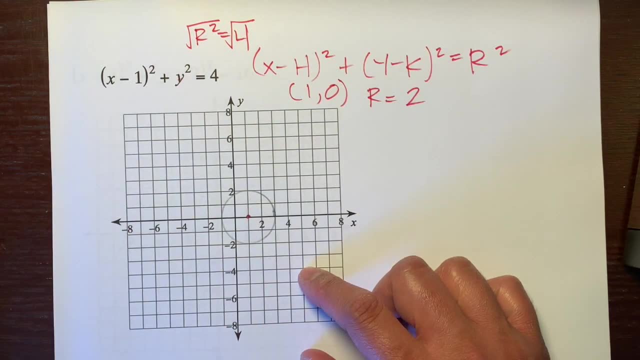 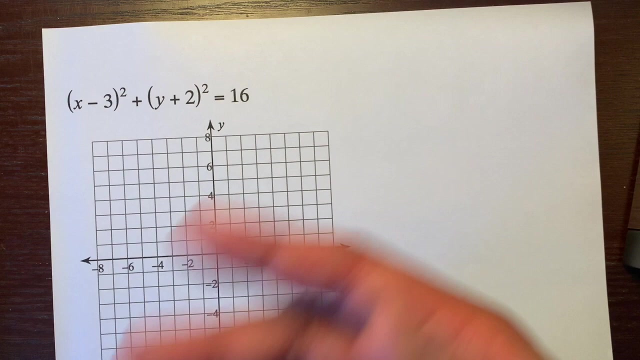 and hey, look at that so that looks better. so, uh, this is two units, the radius there two units, two units, two units, and all of these distances would be two units, the radius is two. so there's the second example, and here is the third and final example on how to graph a circle. so 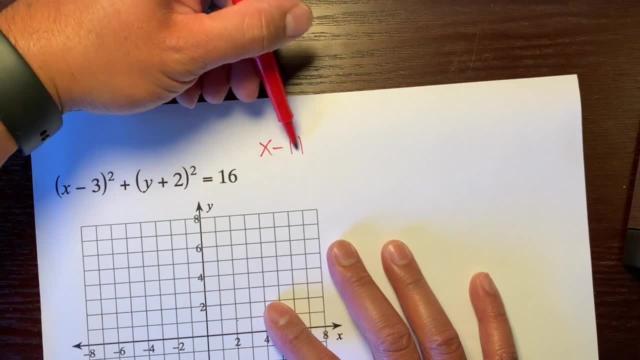 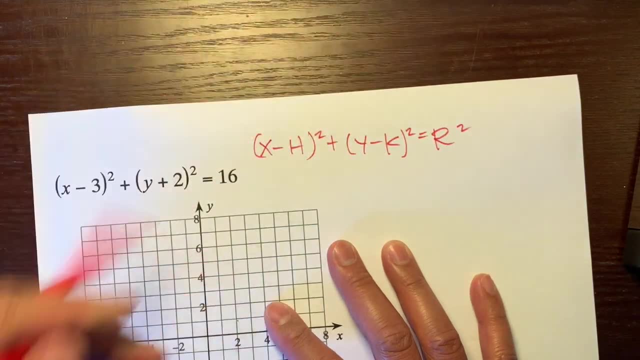 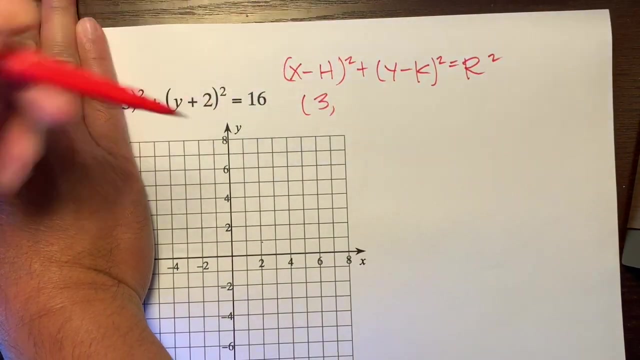 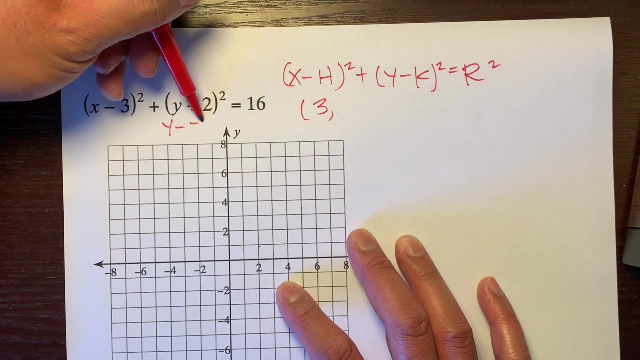 x minus h squared plus y minus k squared is equal to the radius squared. okay, so we're gonna ignore the x minus. so our center would be three comma. now, if you look at this, there is no minus. so we're gonna create that minus by writing y minus negative, two squared. okay, this is the same thing. two negative make. 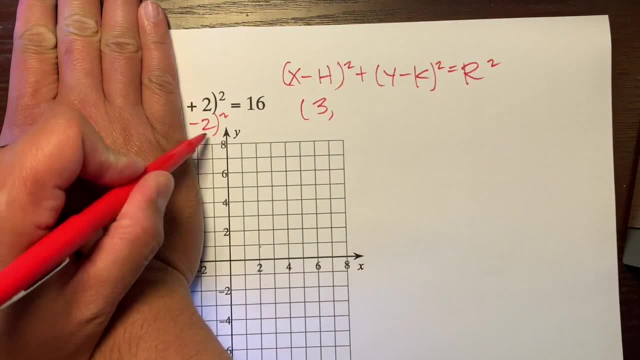 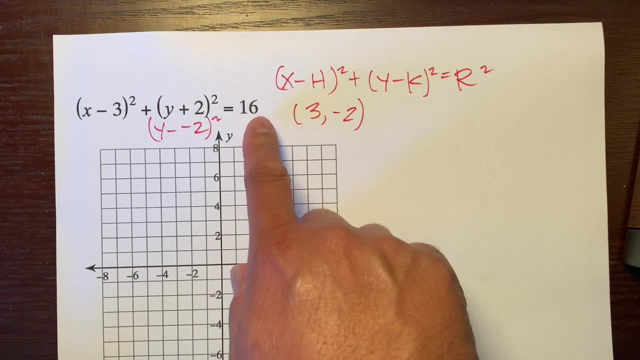 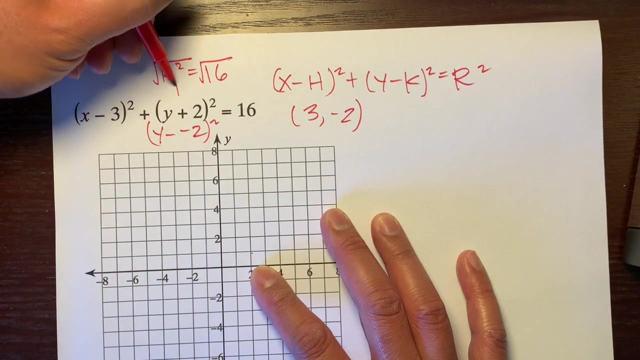 a positive and we'll ignore that y minus and this will be our y value for the sensor. so three negative two. and to get our radius we'll just write: R squared is equal to 16.. We'll square root both sides, so R is equal to four. 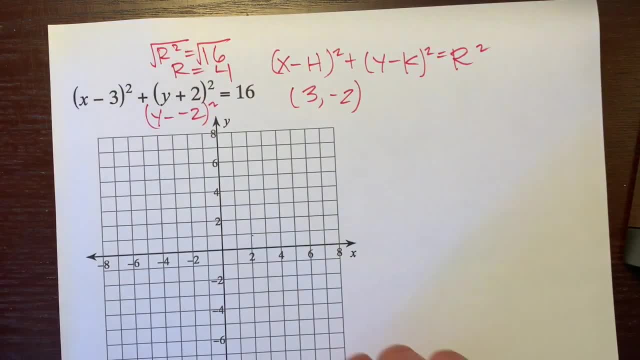 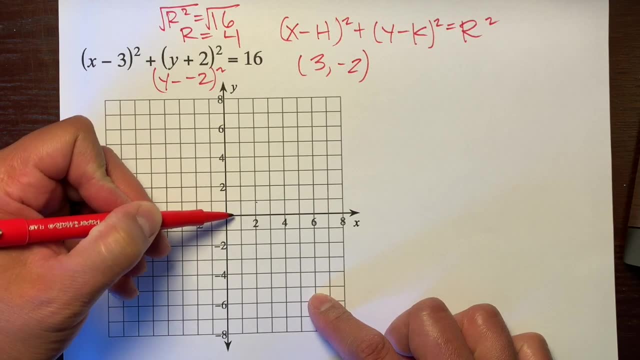 So there's our radius, there's our center. So let's find three, negative two. So we'll start off at the origin: zero, zero. We will shift to the right three units: one, two, three, And we will shift down two units. so one, two.